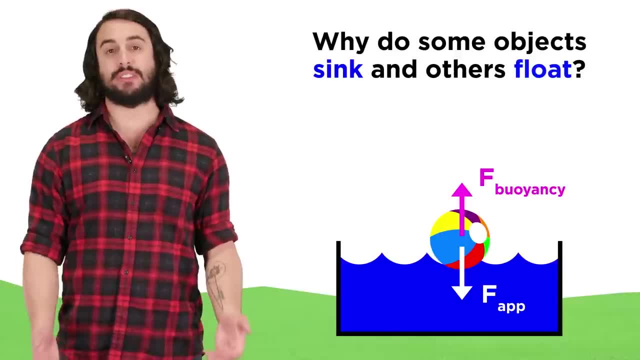 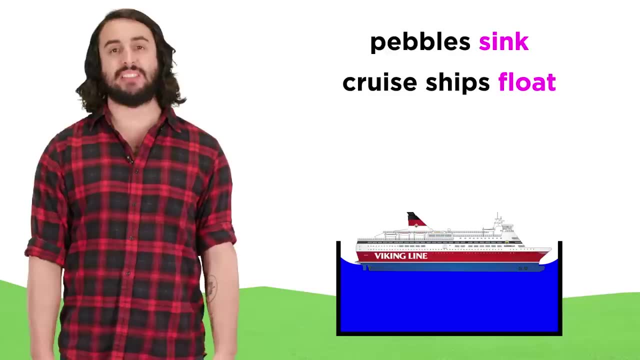 But exactly how strong is the buoyant force, and why do some objects sink while others float? It can't have to do with size, because a tiny pebble will sink while a massive cruise ship will float. The answer is outlined in Archimedes' principle. 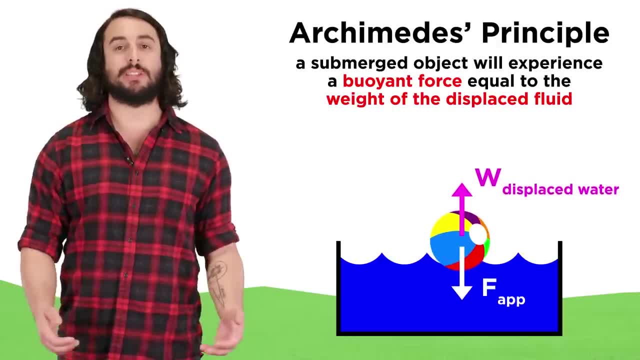 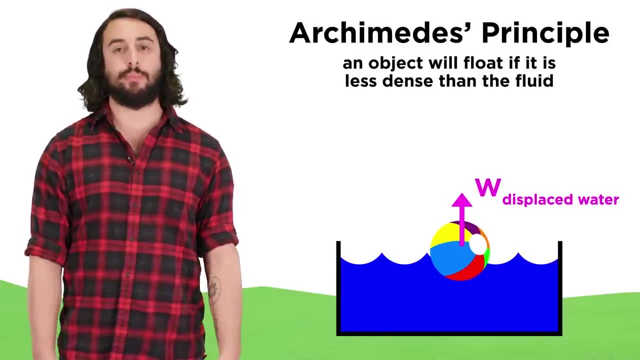 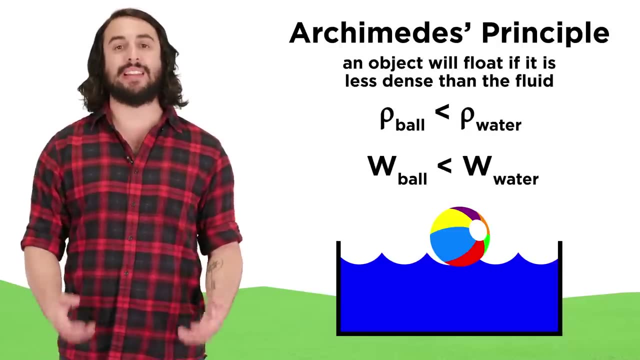 This states that any object submerged in a fluid will experience an upward buoyant force equal in magnitude to the weight of the fluid that is displaced. In other words, the buoyant force will support an object if it is less dense than the fluid, because the weight of the object will then be less than the weight of an equal volume. 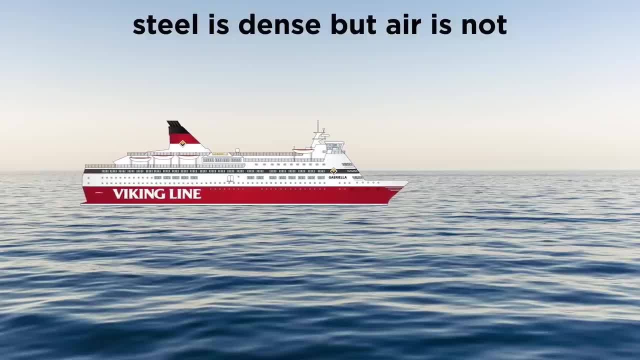 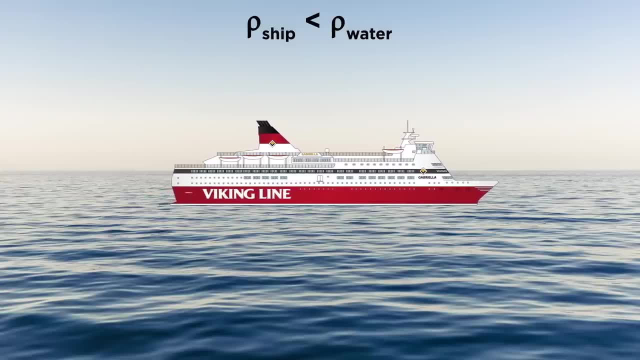 of the fluid. This is why a cruise ship floats in the ocean. Steel is very dense, but the air in all the cabins is not, so overall, the ship is less dense than water If you crushed the ship up into a ball of equal mass, thus eliminating all the air. 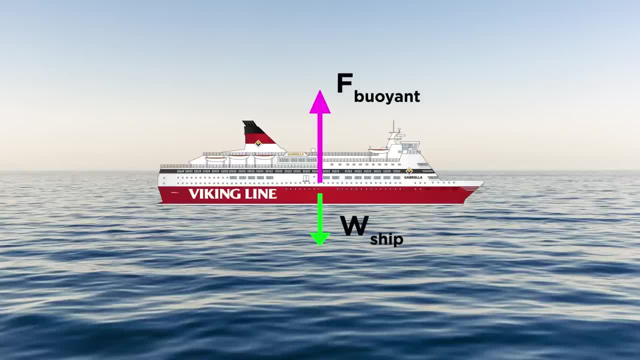 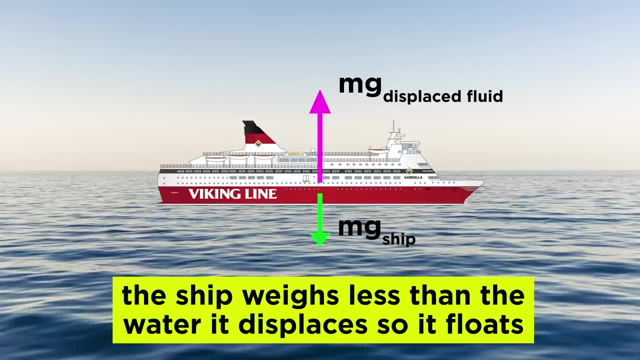 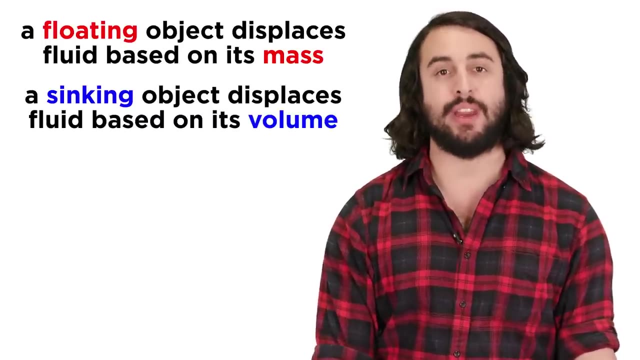 it would definitely sink. In this way, the buoyant force can be expressed as the gravitational force of the displaced fluid, which is equal to the mass of the displaced fluid times acceleration due to gravity. A floating object displaces fluid based on its mass and a sinking object displaces fluid. 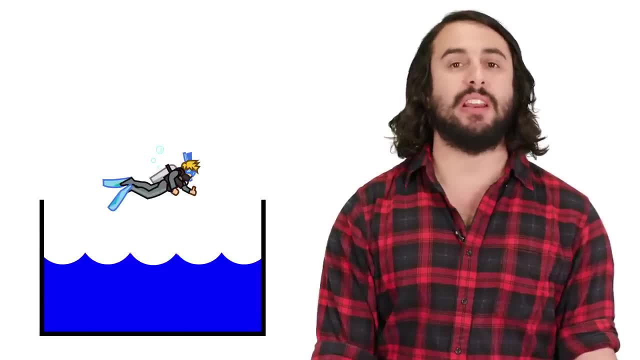 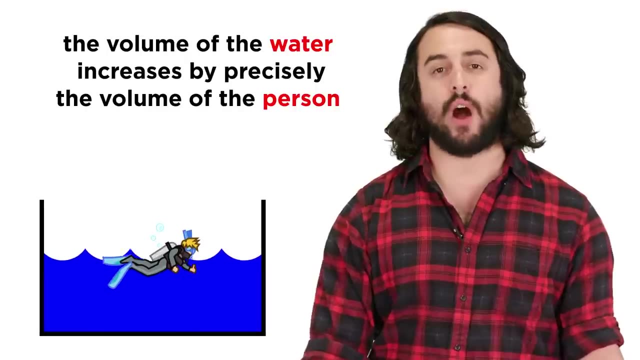 based on its volume. So, apart from the buoyant force, Archimedes was also the first to understand that when an object, like a person, is submerged in water, the volume of the water displaced must equal the volume of the object submerged, regardless of its shape. 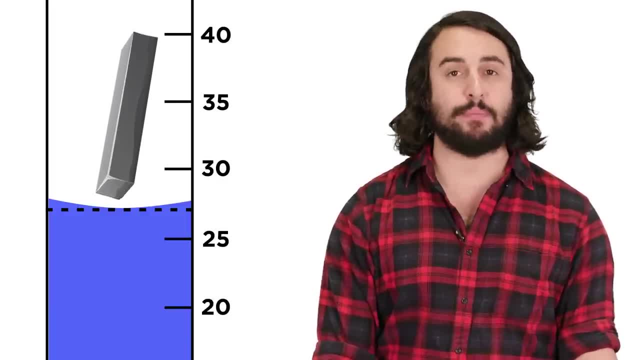 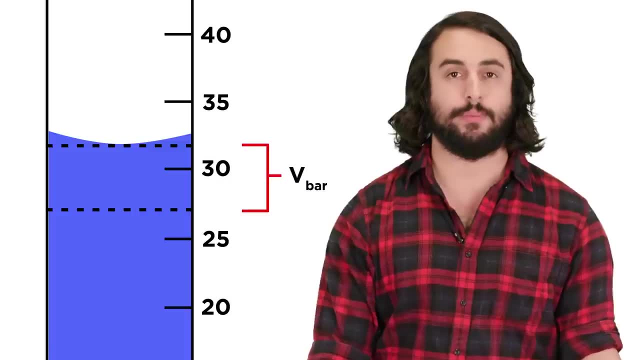 Any object with a volume of five milliliters when fully submerged will cause the water level to rise in this graduated cylinder to a reading of five milliliters more than before. This is an impressive insight for someone from ancient Egypt. I hope you enjoyed this video. 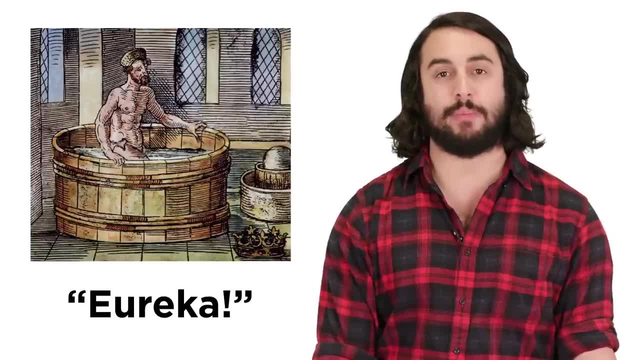 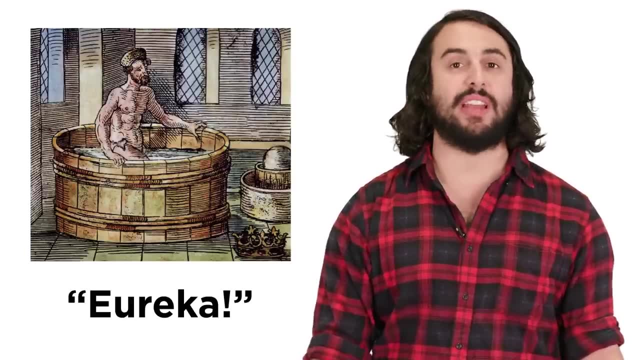 Let's take a break, and then we'll go to the next topic on the subject, which is why Archimedes famously jumped out of the bathtub shouting Eureka, meaning I have found it. This is an exclamation that will forever be associated with scientific discovery.